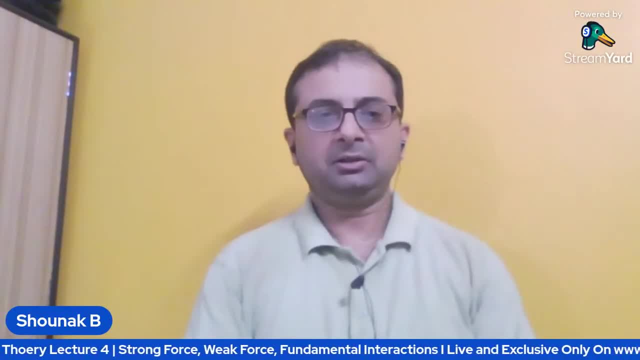 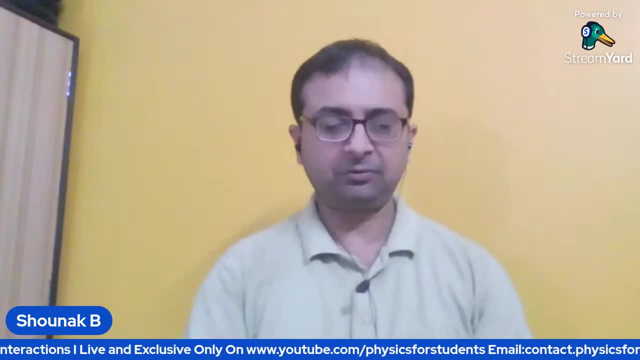 Very good evening and welcome to lecture number four, And I'm extremely sorry those who have watched my earlier lecture, for there was an audio problem, So I am again doing this live streaming because I understand. the problem was that as soon as I'm removing myself and 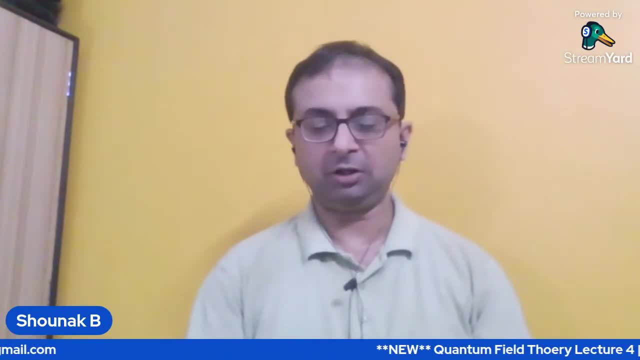 showing the entire slide. there is actually a problem with the audio. So welcome to lecture number four of quantum field theory. Now, those who have seen my lecture earlier- part one, part two and part three- you have seen that these lectures were primarily started with the 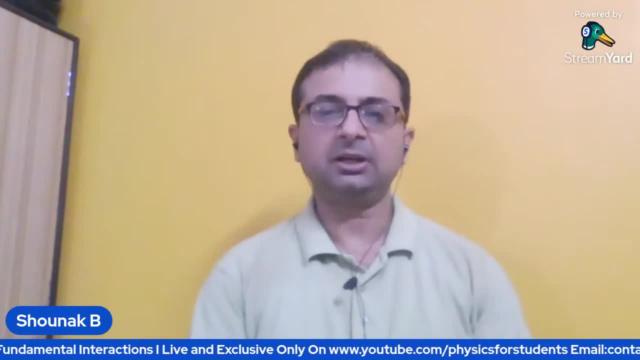 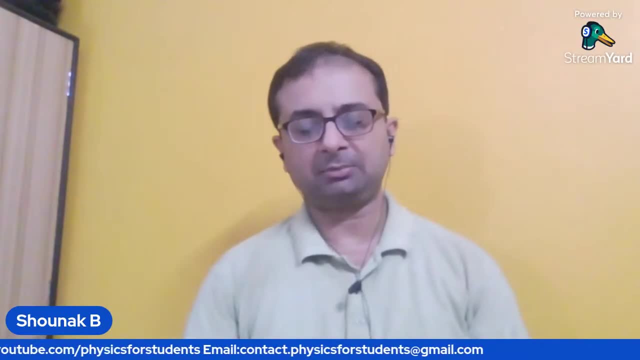 history of quantum field theory. why quantum field theory is required. what is the need of quantum field theory Without quantum field theory, what were the problems? Quantum electrodynamics, quantum chromodynamics, the quarks, the leptons. Most importantly, we have 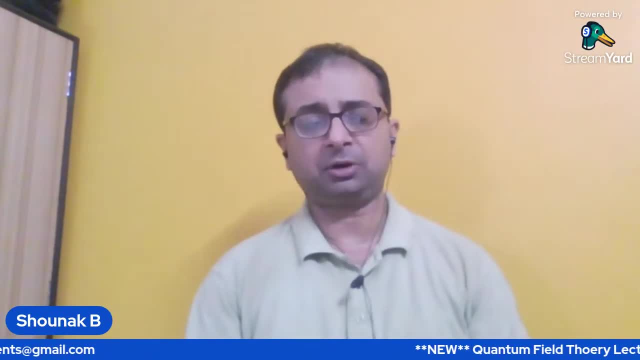 dealt with Schrodinger's equation, the classical limitation of Schrodinger's equation. Thank you for watching. Welcome to Sushil Gunratne, who really appreciated my derivation of the Schrodinger's equation. It actually showed that why Schrodinger's equation is unable to show the spontaneous 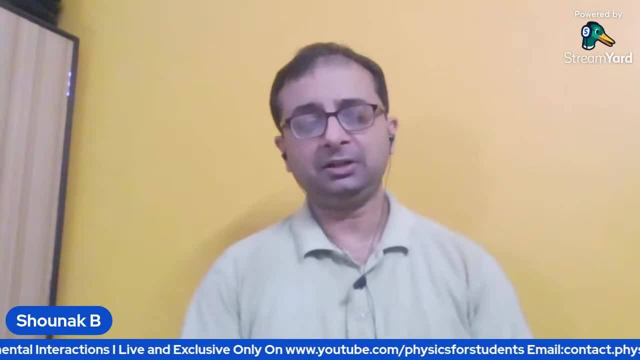 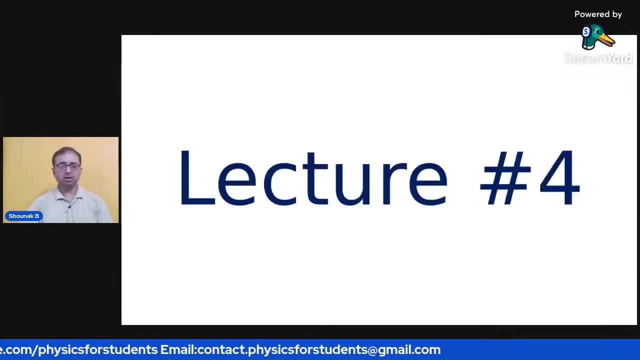 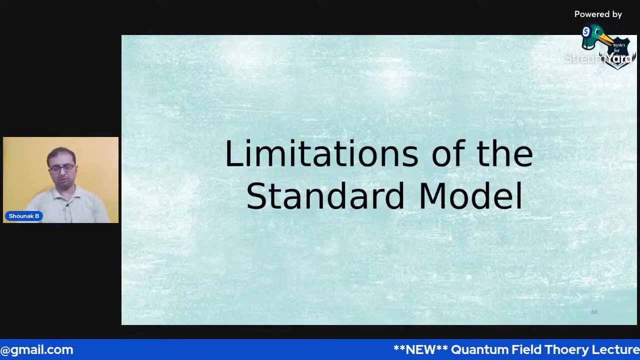 emission, the limitations, as the radius of a spherical mass of electrically charged goes to infinity, and different other things. So in today's video, today's lecture, I would be explaining a little bit upon the what we call the limitations of the standard model. Now, 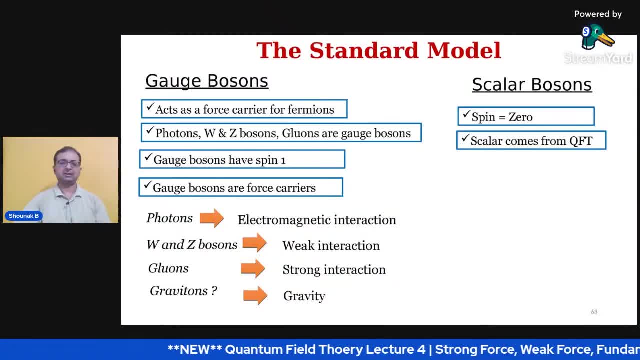 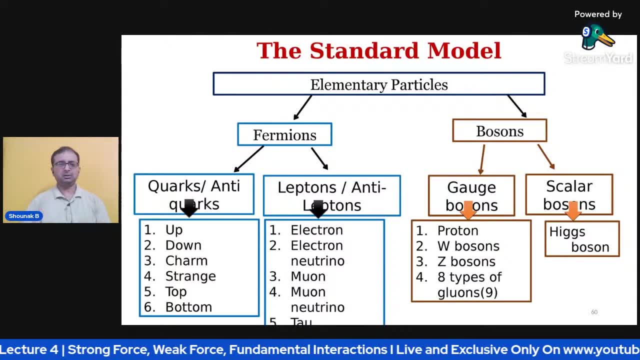 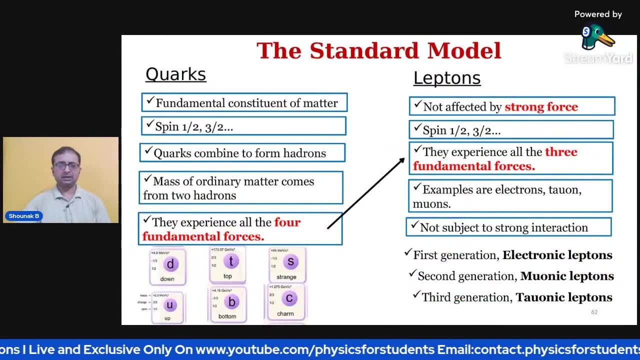 if you go back to my previous videos, these are the slides where I have explained basically the standard model, which explains everything, starting from the elementary particles to quarks, the up, quark down, quark charms, protons, bosons, everything. Although standard model quarks, 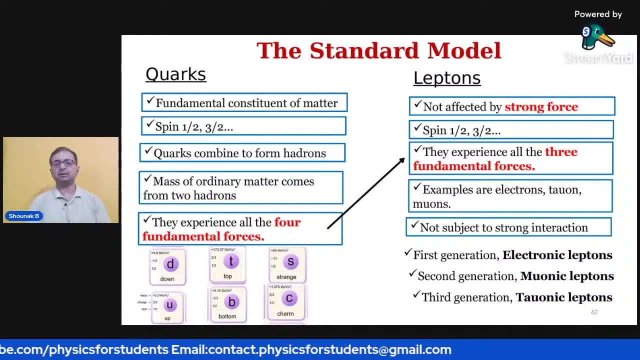 leptons, etc. they actually define and make understand of all the other forces. So in this case I would say there are still certain limitations of the standard model. but I would say that there are still certain limitations of the standard model and I would say that there are. 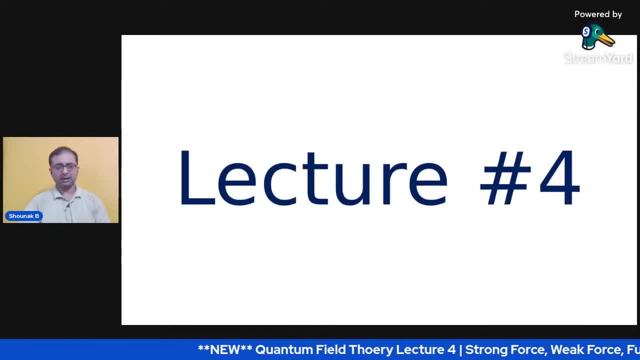 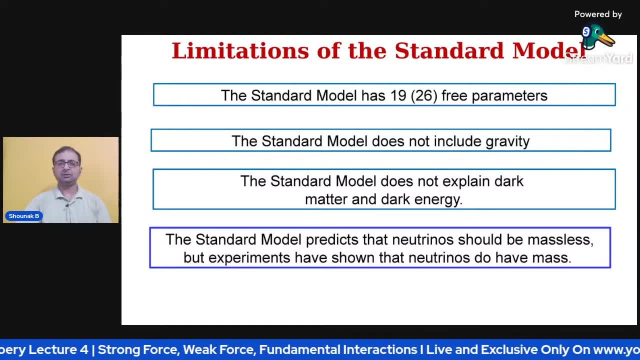 still certain limitations of the standard model which I would definitely like to explain in today's lecture. So first of all, let us understand what are the limitations of the standard model And in this case I would say the basic first limitation is what is called 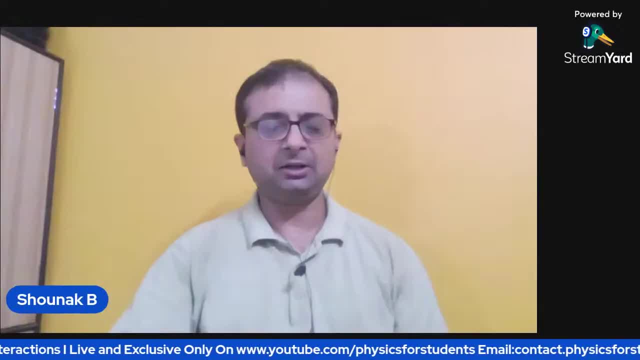 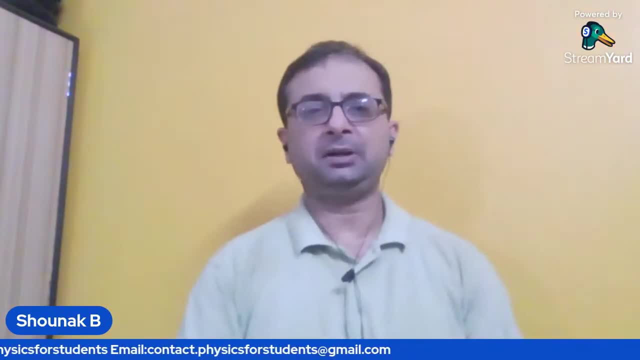 is a free parameter. Now, first of all, what I would like to explain to you is that: what is actually a free parameter? Now? say, for example, in case of defining a particular mathematical model. we sometimes do certain things. we can make a model which can be. 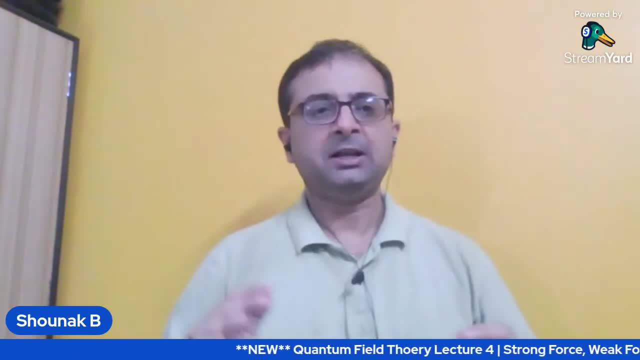 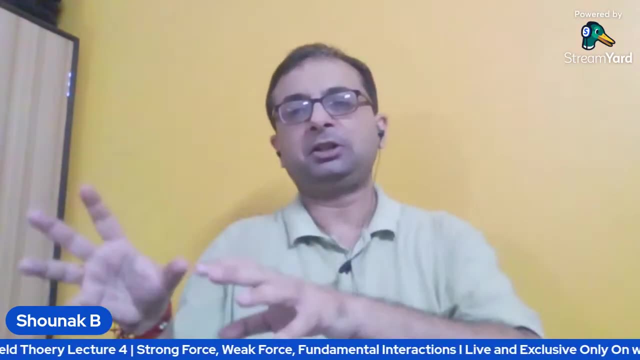 experiment which can be measured experimentally. Okay, So, for example, we want to develop a motion of a projectile. So we start with certain assumptions, right, The projectile, such as that it is moving in a vacuum, it has got a velocity, there are other forces like gravity, etc. And then 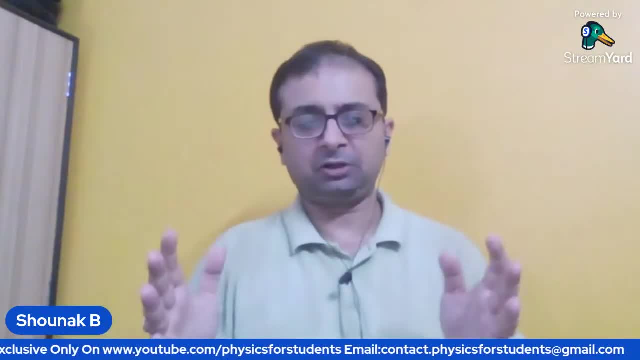 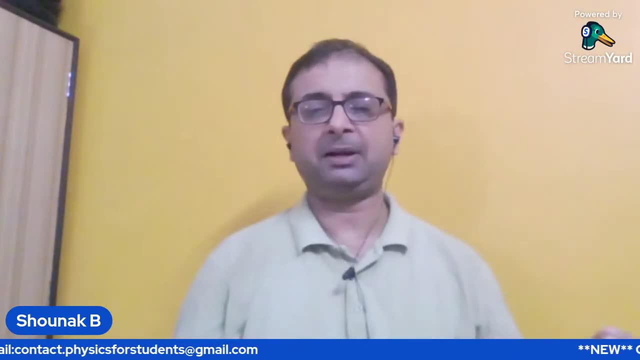 you can use these assumptions to write down a set of equations that describes the motion of the projectile. Now, these equations- whatever, x, y, z, etc. whatever it will happen- will contain some unknown quantities. So we can write down a set of equations that describe the motion of the projectile. 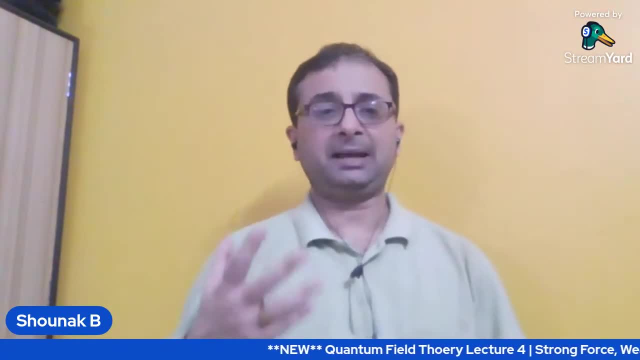 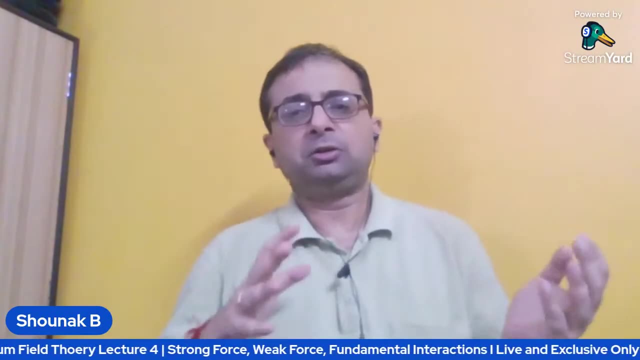 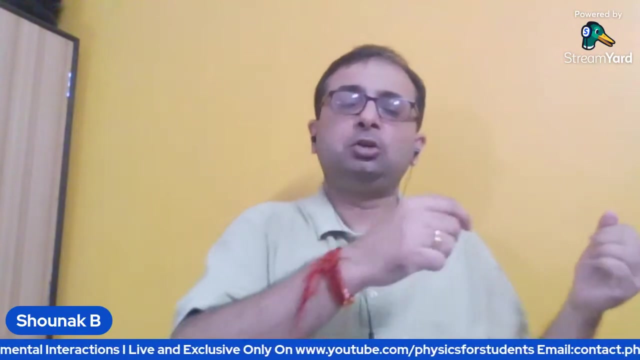 And such as initial velocity of the projectile, its mass, etc. Now, these unknown qualities are basically what are called free parameters. Okay, So to determine the values of the free parameters, what we need to do? we need to do an experiment. So, for example, to measure the initial 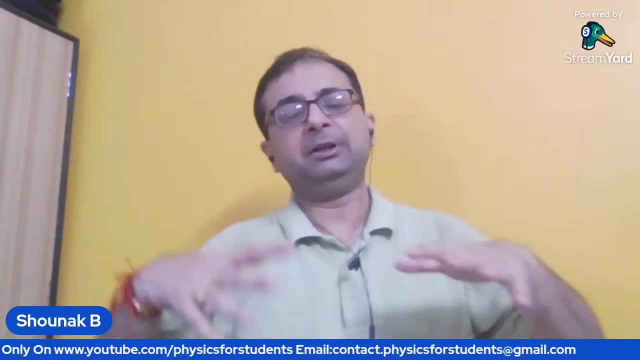 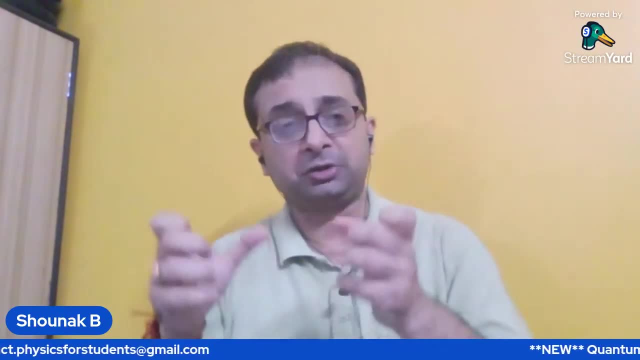 velocity of the projectile which is being fired from a gun and measuring its speed with the radar, etc. So once we determine the values, that means the equation which contains those unknown quantities and the free parameters, then obviously the mathematical or the theoretical model of the 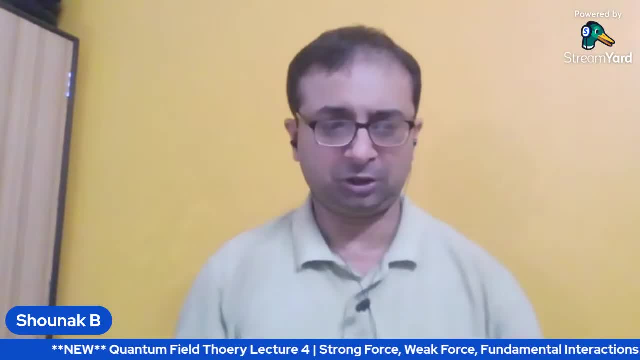 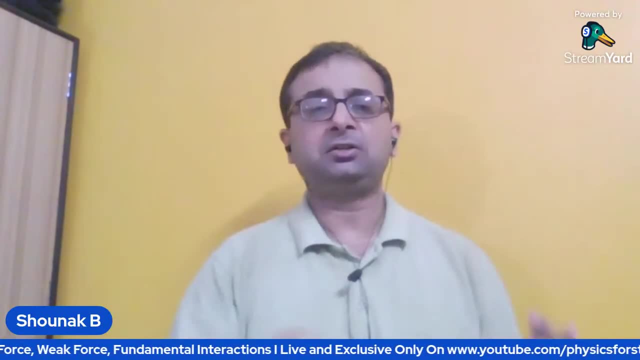 projectile or whatsoever can be given any set of initial conditions. So free parameters are essentially tools for developing and testing physical models And it is important to be aware that free parameters it has got certain amount of limitations. Okay, let me go back to my slide. 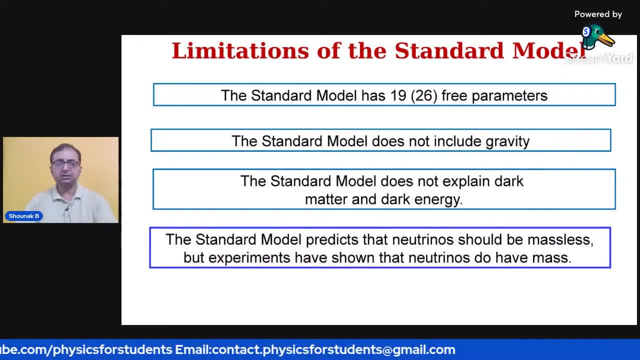 now and things would be easier now. So, yes, you see, some people say that there are 19,. some people say that there are no free parameters. doesn't matter, But what matters is that these free parameters provides a kind of a limitation for the standard model. First of all, as you can see, 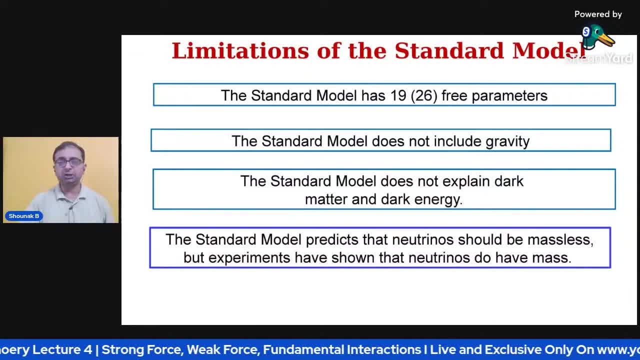 that in case of a free parameter, especially the neutrinos, they have a mass. If you have attended to my earlier, you know YouTube live with Dr Jessica, who has exclusively spoken about neutrinos, that neutrinos do have a mass, etc. So neutrinos do have a mass, But the problem is 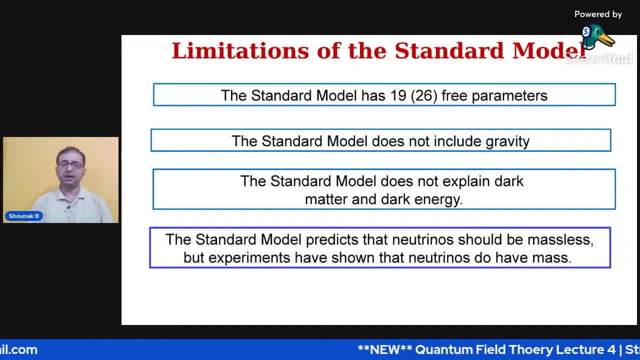 the standard model doesn't yet define what is that neutrinos mass, Although experiments, as I told you, shows that neutrinos do not have a mass. So standard model predicts that neutrinos should be mass but massless. but experiments have shown that they do have a mass. So here is a contradiction. 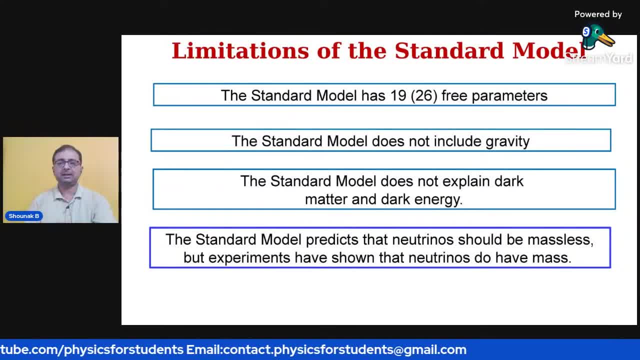 Standard model shows that there should be massless, but experiment shows that neutrinos do have a mass, So the free parameters are not properly defined And that is basically a problem with the standard model. Also, let us remember that the standard model does not include gravity, So gravity is one of the four. 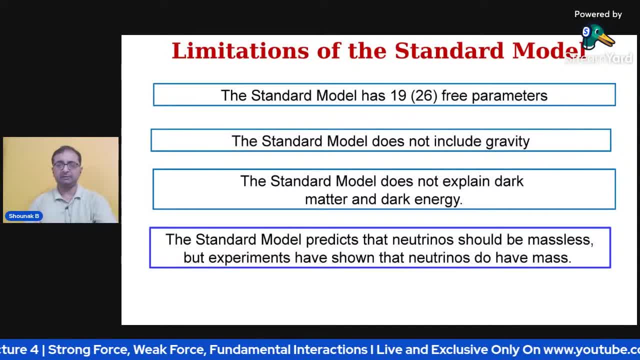 fundamental forces and standard model does not include gravity, which we are still studying. Standard model also does not include the definition or explanation of dark matter and dark energy And we know there are a lot of researches in cosmology etc going on in dark. 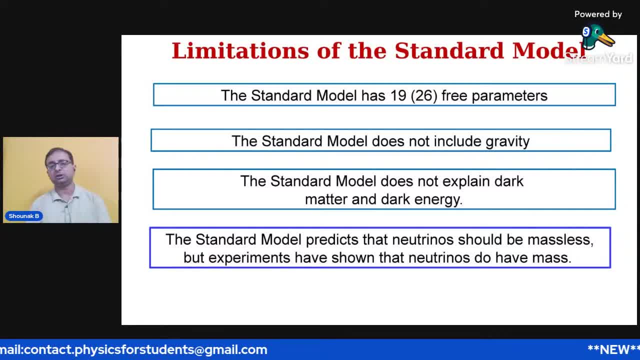 matter and dark energy, which makes up 95% of the universe, And so you know there are a lot of engineers. but the standard model does not provide anything. So it does not include gravity, it does not include free parameters, it does not explain dark energy And, as I told you that it should be, 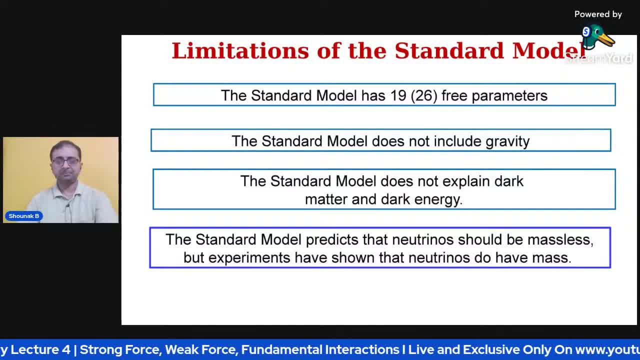 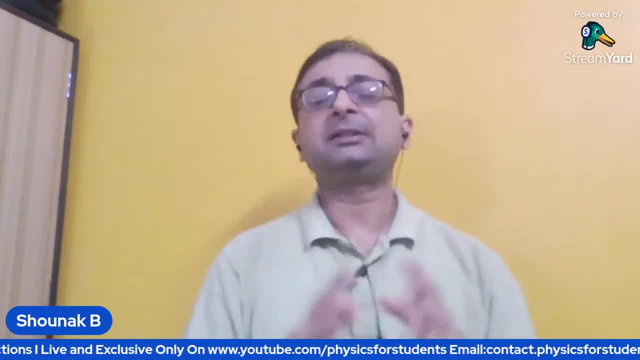 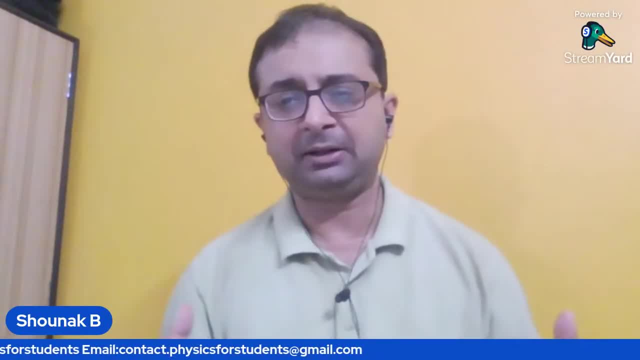 massless, but it should define that doesn't have a mass. So but what? I would say that despite all its you know kind of limitations etc. A standard model in particle physics is something which will accurately describe a wide range of experimental data. However it is, 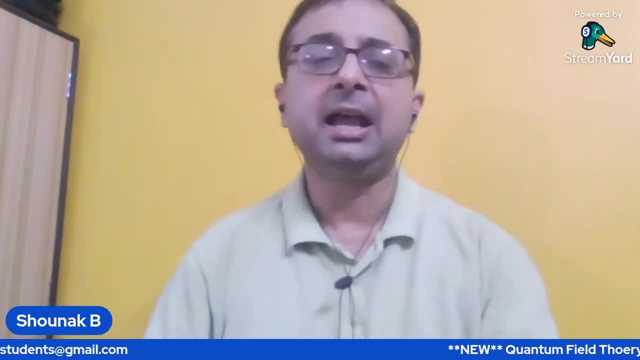 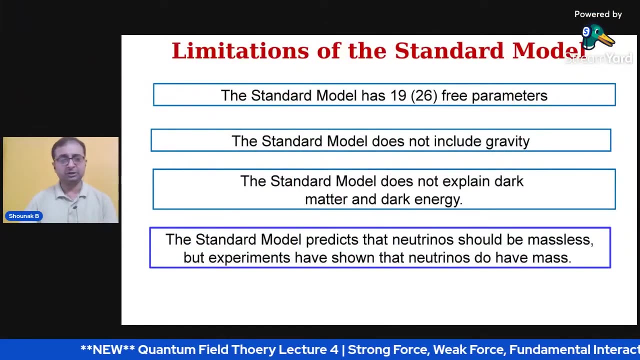 clear that the standard model is definitely not a complete theory, And with a new physics or a new model in which these neutrinos, massless parameters, etc. can be defined using the standard model. Okay, so, having laid this kind of a definition, I would come to what is called the 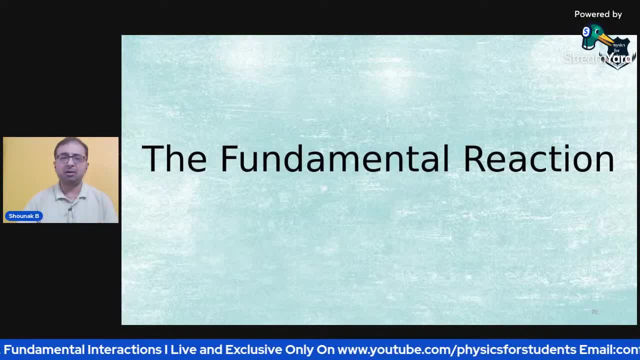 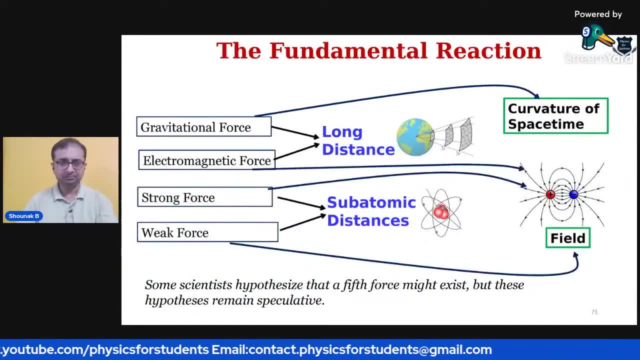 fundamental interaction, Fundamental reaction, in the sense that all the major forces of nature, whatever that we are dealing with, can be explained with this: fundamental forces. Okay, just let me check in whether my audio, I think, is now working. nice, If somebody is watching, can you just put it? 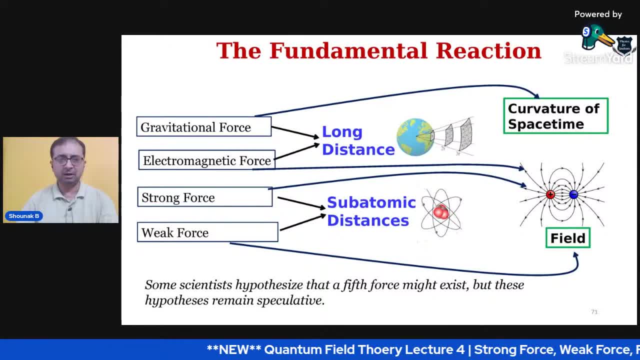 in the comment box that, whether the audio part is now, the audio is going nice and fine. Okay, in the chat box, if you can just put it to me right, Okay, so what we see from here particularly is that these are the four forces of nature. 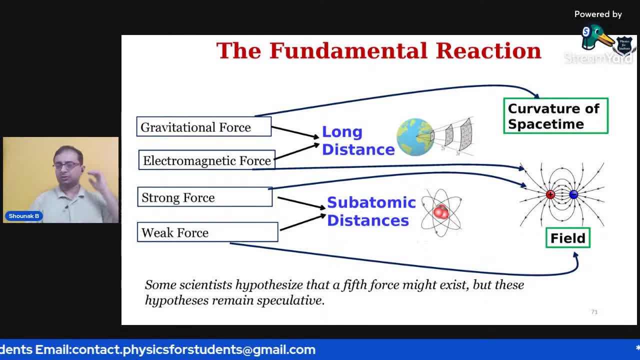 So we see that gravitational and electrical magnetic interactions with produces significantly, I would say, long range of forces whose effects can be definitely seen in everyday life. right? So you see the gravitational forces, the curvature of space, time it happens and it has got a long distance. electromagnetic force: 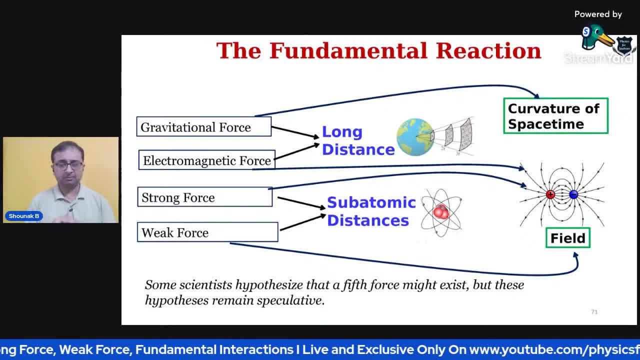 also happens with a kind of a field, as I've shown in the slides. the strong forces, these are the subatomic particles and the weak forces also. So each of these need known fundamental interactions can be described mathematically. So we see that the strong forces, these are the subatomic particles. 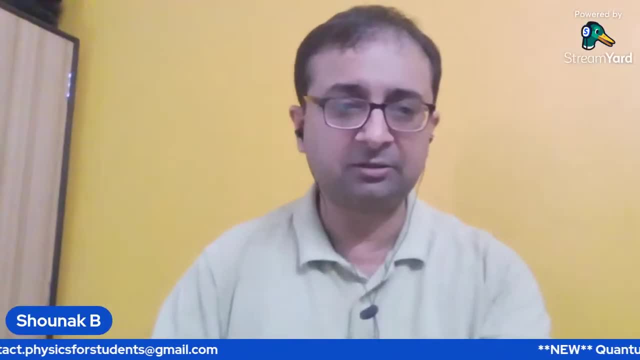 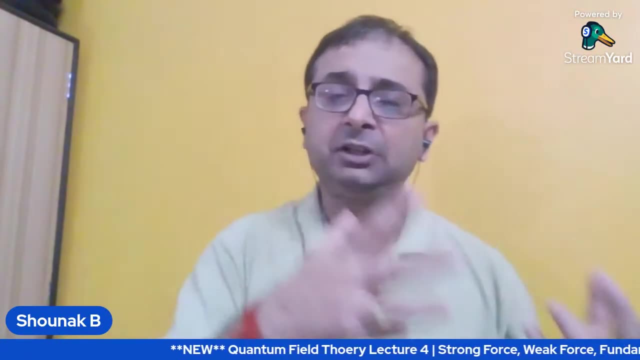 can be described mathematically as a field. This is- this is very important. Each of these fundamental interactions can be described mathematically, which is called a field, and the gravitational force as attributed to the curvature of space time is described in Einstein's general relativity, The 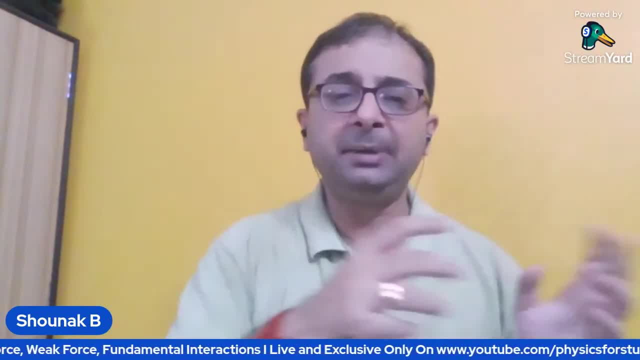 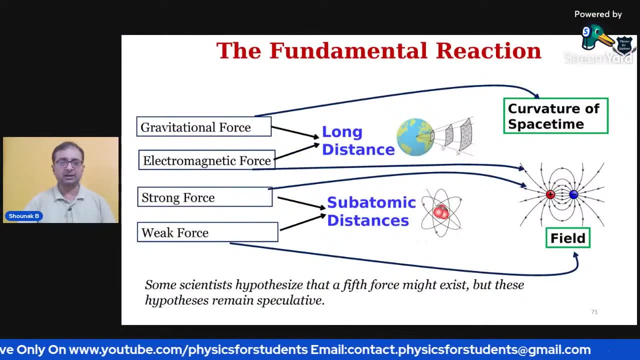 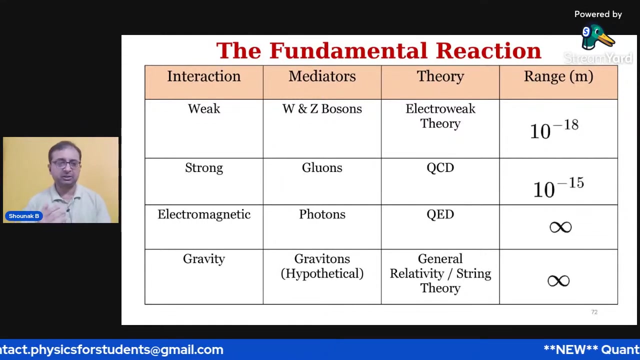 three other discrete quantum fields. and then interactions are mediated by the elementary particles and defined in the standard model. And now we are going to see that what are those particles and how do they interact in the next part. So here you can see that the weak interaction, that the weak force, the strong force, the electromagnetic 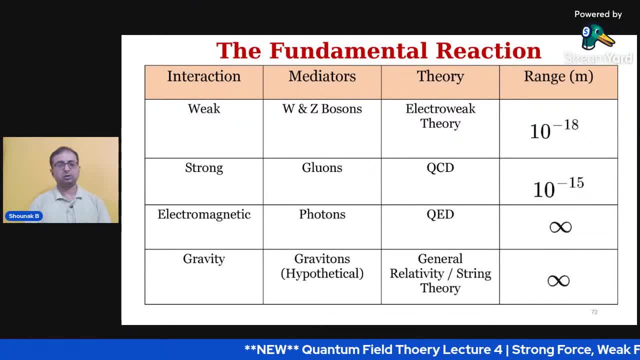 and the gravity. So these are the mediators, W and Z bosons, the gluons, the protons and the gravitons. So these are the electroweak theory, quantum chromodynamics, quantum electrodynamics and generativity, or the string theory which is being taught Now in terms of gravity, to 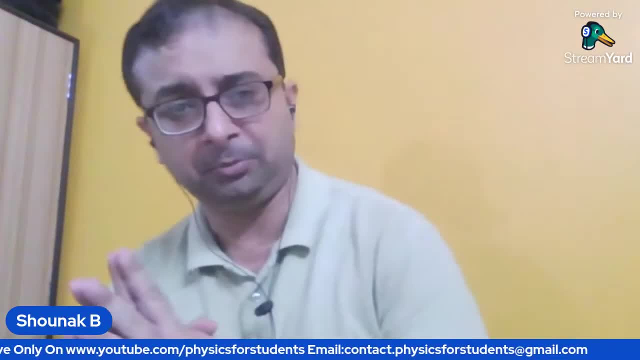 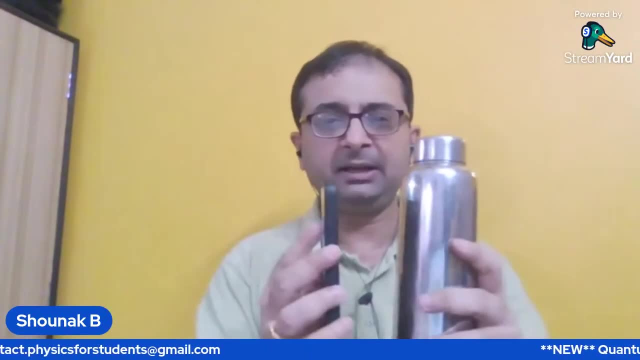 be taken as weak force. here I have got a point to make Now. considering, say, for example, this is a bottle and this is a mobile, So in case we are bringing things together to each other, we will see nothing is happening. 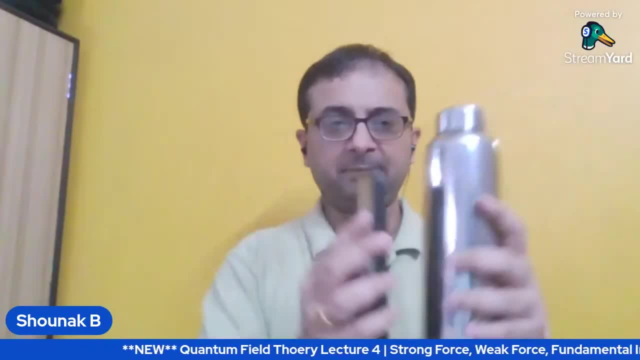 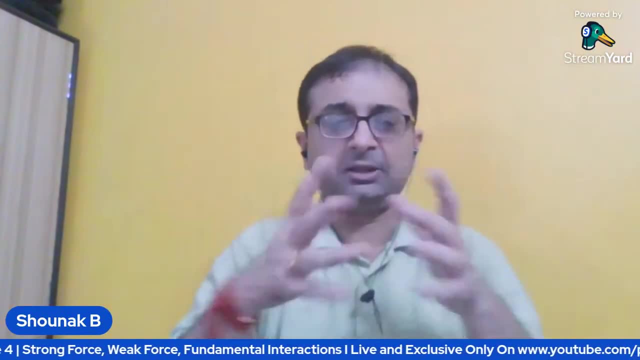 Still, these are. this is a big mass, and this is a big mass. We are bringing things together but nothing is happening. But in case of an electromagnetic or a weak force, if you bring things together, it causes a problem. It causes. 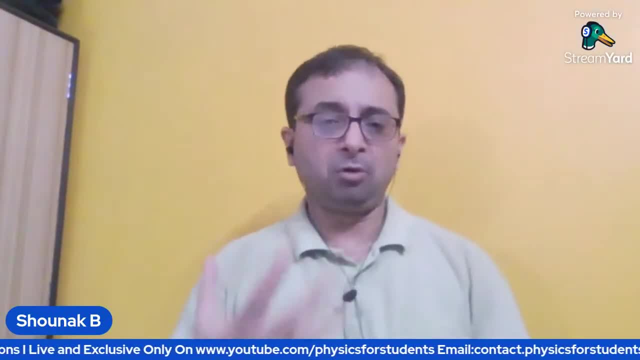 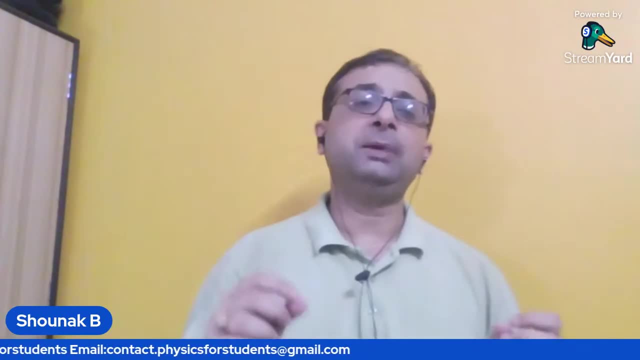 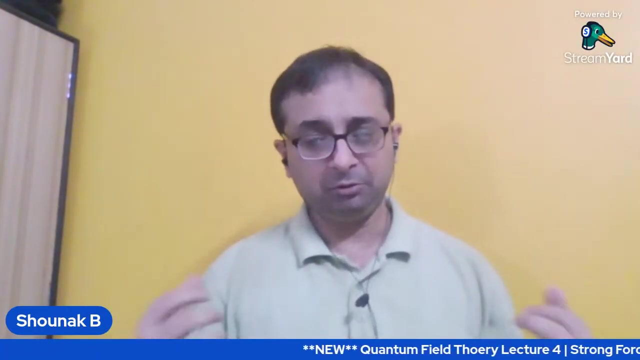 a kind of a reaction. So, what is more important, that you need to understand that gravitational force is called weak also for another reason: that in order to measure the curvature of space-time, we require a huge mass. We require a mass which is as large and as huge as a Jupiter. We require 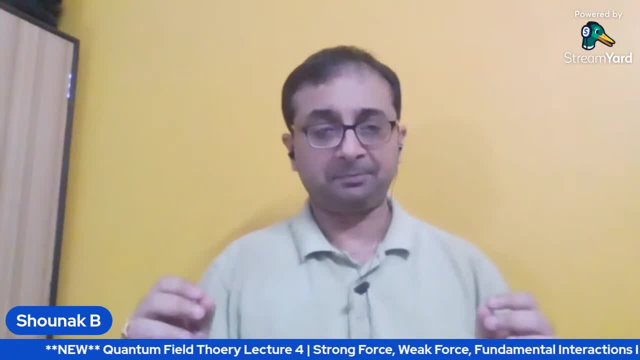 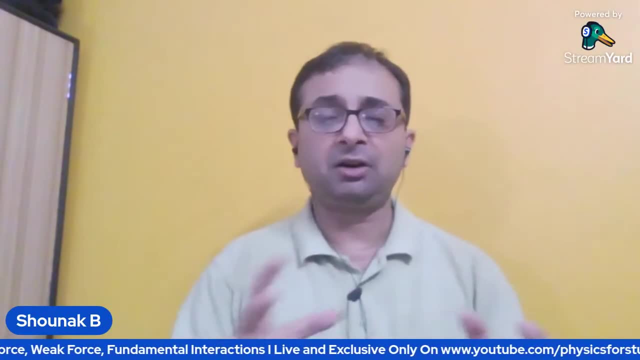 mass as large as a supermassive black hole or something like that. That means it is weak. in terms of what? In terms that only when we get such a huge mass, then only gravity or Einstein's equations will be able to define the space-time curvature, otherwise not. So this is one of the 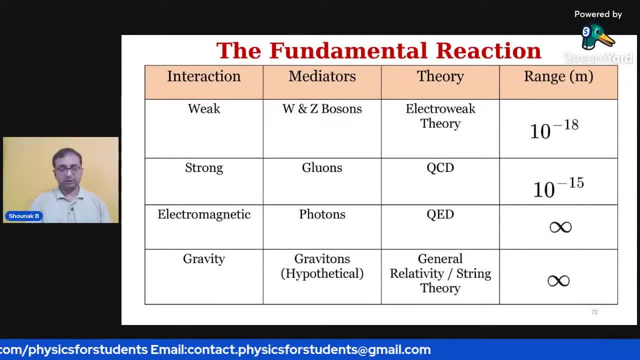 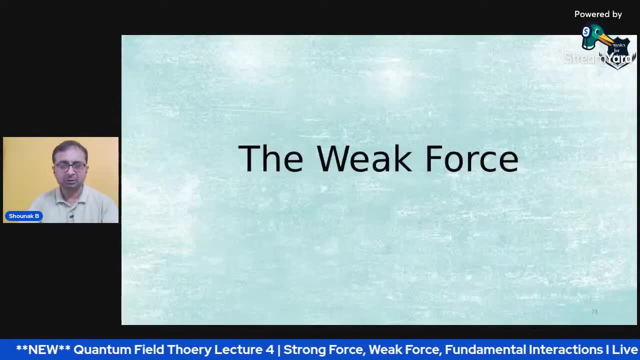 aspects of calling gravity as a weak force. So there's a strong force, there's electromagnetic force and there is gravity. So, taken all these things together, these are actually the fundamental reactions. So the fundamental reactions are very fundamental, which explains everything related to gravity. Okay, so we go from here and we try to understand what is a weak force. So here you can. 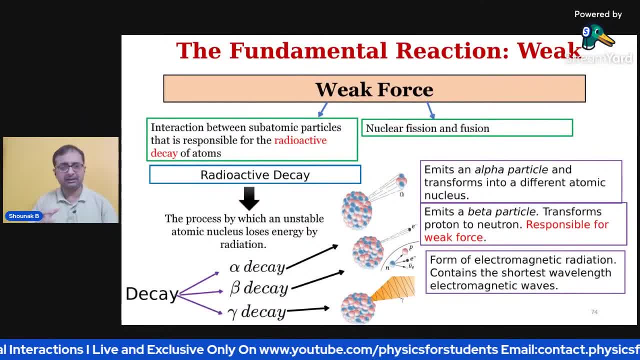 see that weak force is. basically. there are two types. One is the interaction between subatomic particles That is responsible for radioactive decay, and it is also weak force is something which is responsible for nuclear fusion and nuclear fission. Now here is one thing you need to. 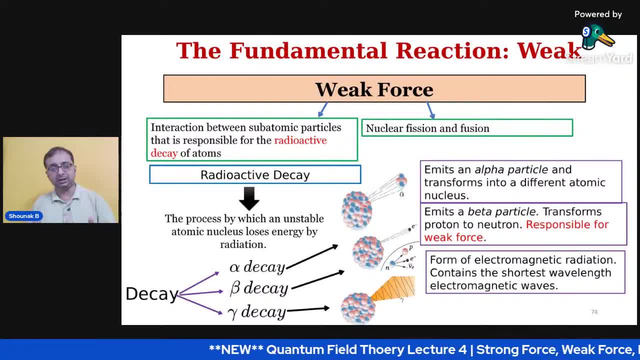 understand Radioactive decay, which is also known as nuclear decay or radioactive disintegration. This is the process by which an unstable, I would say, atomic nuclei loses energy by radiation. It loses energy by radiation So strong and weak force. Weak force is loose, It radiates. 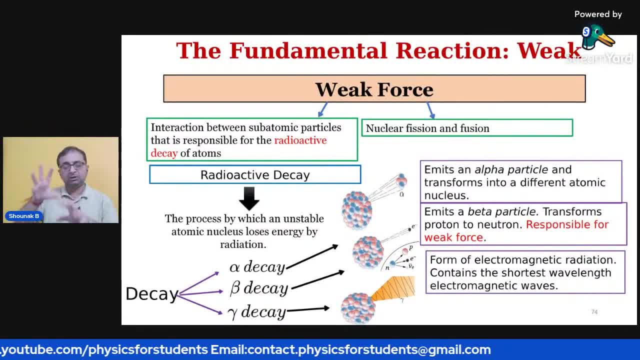 And it gives radioactive decay. Now there are three types of decay, as I have pointed out in the slide, As you can see: alpha decay, beta decay, gamma decay. I will come to those decays later, But remember that the weak force is the mechanism that is responsible for a radioactive, for that. 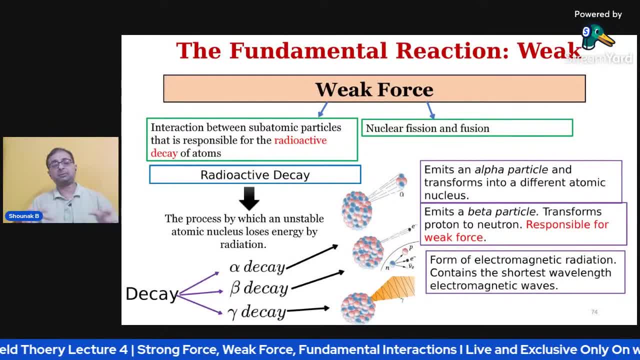 beta decay. So there are other two forces which are governed by electromagnetism and nuclear force, And there is- some people feel that there is- a fourth type of force, which is called, which causes an electron capture, in which basically an atom nucleus and an inner electron, you know, emits from the electron shells. 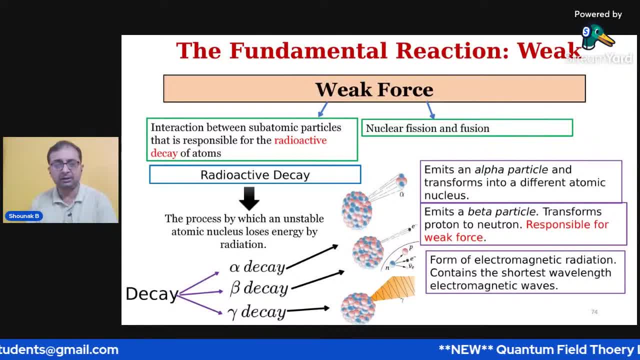 So alpha, beta decay and gamma decay will come to that part later. But it basically emits a part of alpha particle, transforms it into atomic nucleus, It emits a beta particle, responsible for weak force, and forms an electromagnetic electron and it's shorted wavelength. So this is basically what we call is a weak force. 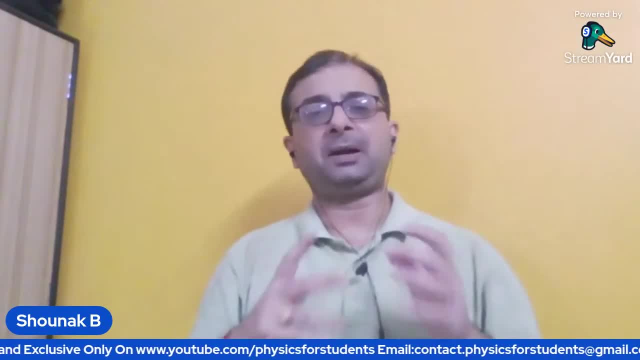 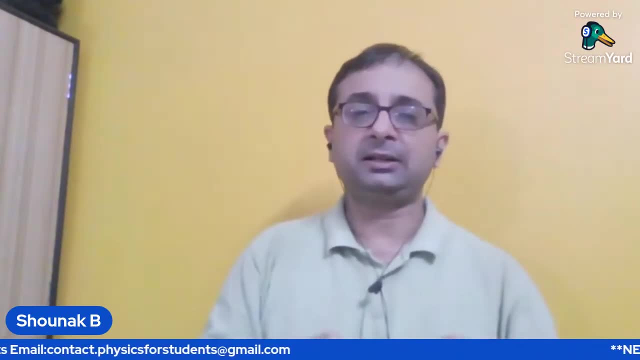 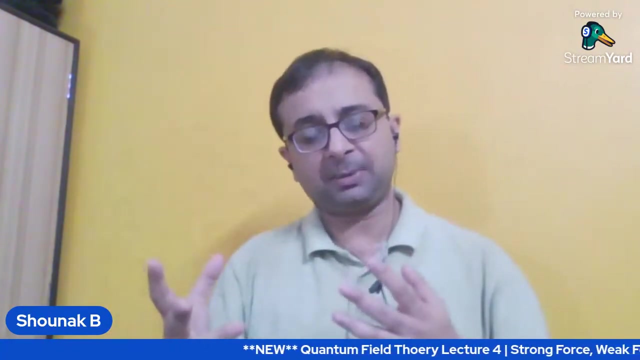 Now you might be wondering that these are Very fundamental in terms of particle physics. But why am I teaching, teaching those things? This is important because we need to understand that until we understand the basics- the particles in motion, their characteristics, behavior, etc. When we move into the Lagrangian and the difficult part of mathematics, things will be much more difficult. 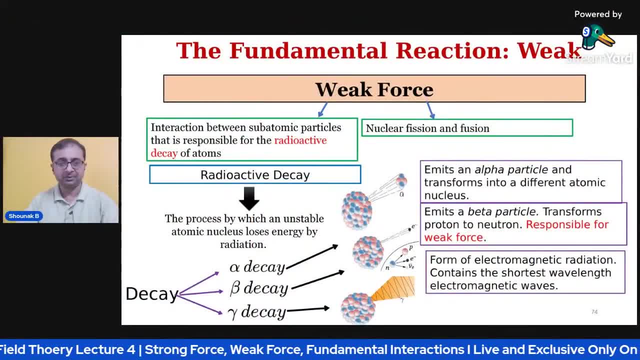 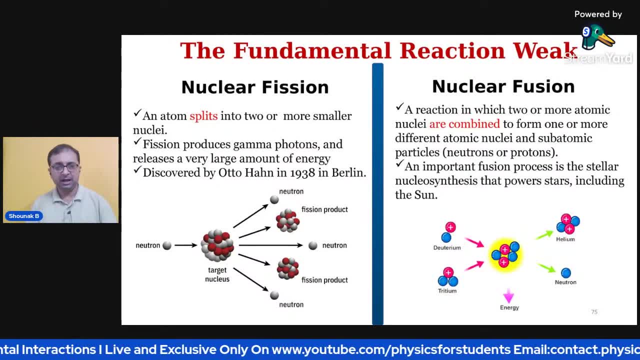 So that is, that is how we make up things. So from here you see, there is a concept which should be cleared up, That is, what is a nuclear fusion And a nuclear fission? So, very simple, fission is somewhere an atom splits up into smaller nuclei, and fusion is a reaction where which two or more atom 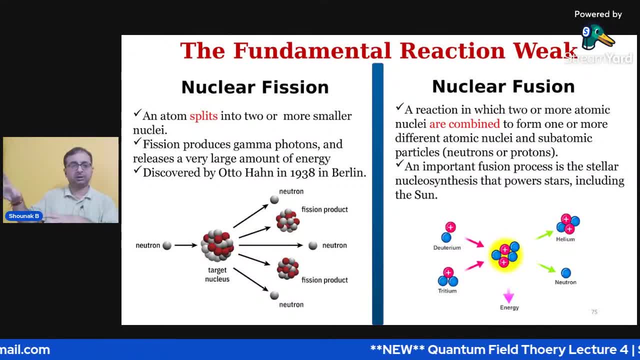 nucleus are combined to form one or more different atomic nuclei. So fission is bad. It actually splits up a nuclear fusion. is you know thinking that? that is why we call all those fusion music and fusion foods? because we are bringing things together. right, We are bringing things together. 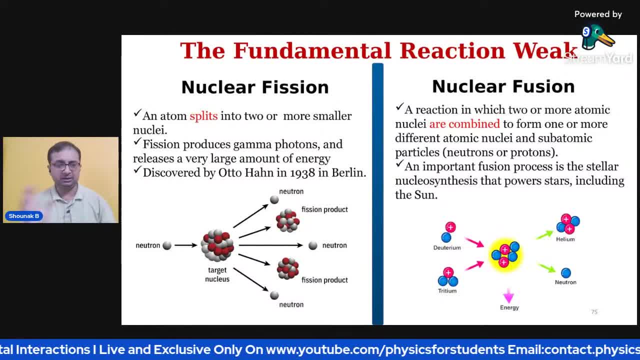 That is why we call it is a fusion, And fission is Basically decaying of those particles. So this is being discovered by Otto Hahn in 1938.. And this is an important fusion because the nuclear fusion actually happens in stellar nuclear synthesis in terms of stars. 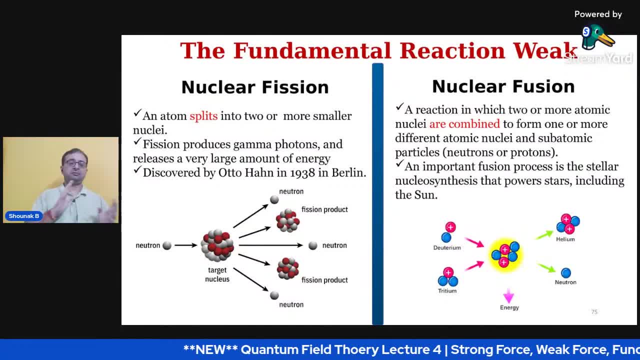 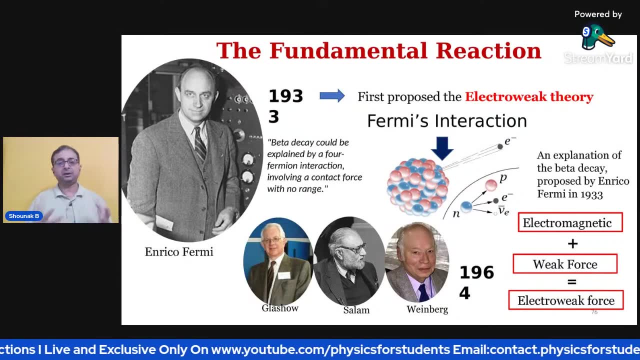 etc. So do have a clear understanding of a fusion and fission. So fission is something which breaks up into smaller, smaller nuclei, and fusion is something which brings things together. OK, Here is And something very important. So it was Enrico Fermi, or Fermi interaction, which is an explanation of the beta decay. 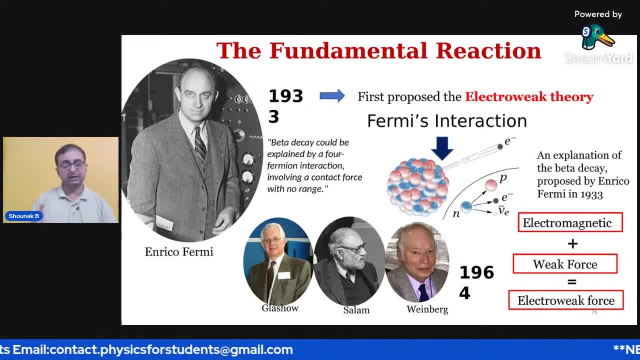 So remember that it was Enrico Fermi who first proposed the electroweak theory, although later it was united by Abdu Salam Steven Weinberg model. But it acted as a kind of a precursor to the fundamental fundamental reaction. So Enrico Fermi's interaction is an explanation of the beta decay, which was first proposed in 1931 by 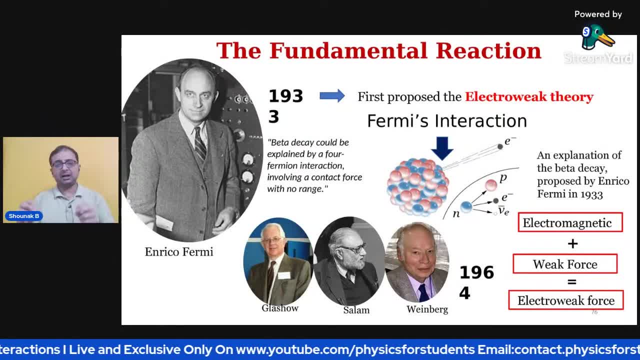 Enrico Fermi. The theory actually posits that four fermions directly interact with each other, And Fermi was the first to introduce this coupling in his description of beta decay Right. Just hold on for a second. Why So You? 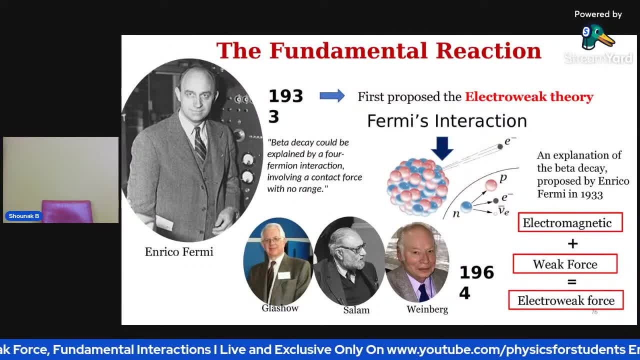 Can Have The Or This Situation Right. So this was that And later, as you can see, these three gentlemen of the salam, Stephen Weinberg and Sheldon Glashow, actually united this And it was awarded Nobel Prize in 1979. 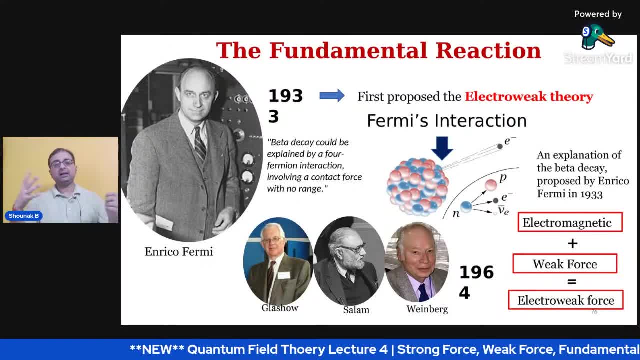 And for their contributions to the unification of the weak and electromagnetic interaction of elementary particle, which is known as the Weinberg Salam model. So this was the first unification. unification, it was done, but let us remember, prior to this interaction of this theory, it was: 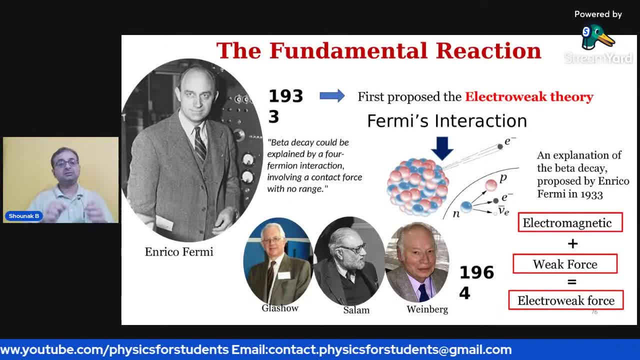 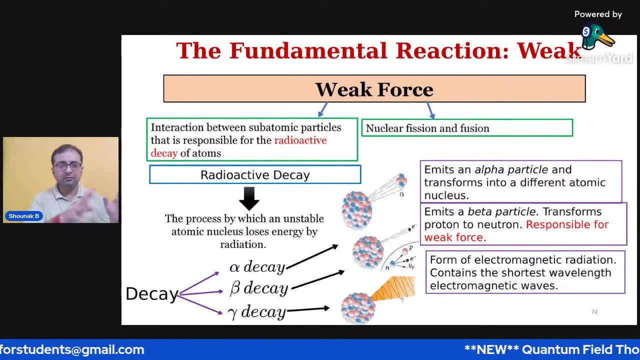 Enrico Fermi who first proposed the electroweak theory, and it was through Fermi interaction that the beta decay comes into play. and now, if you go back to my this slide, you can see here weak force actually is responsible for the radioactive decay, and this radioactive decay consists of three. 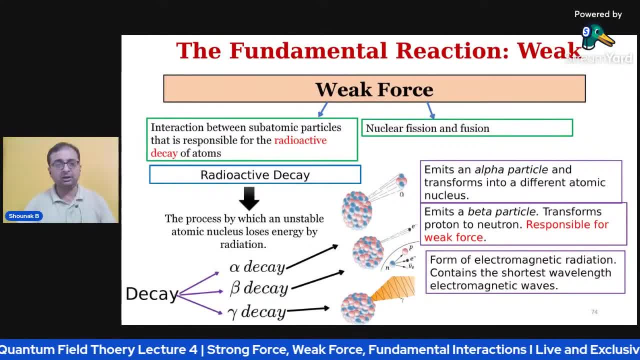 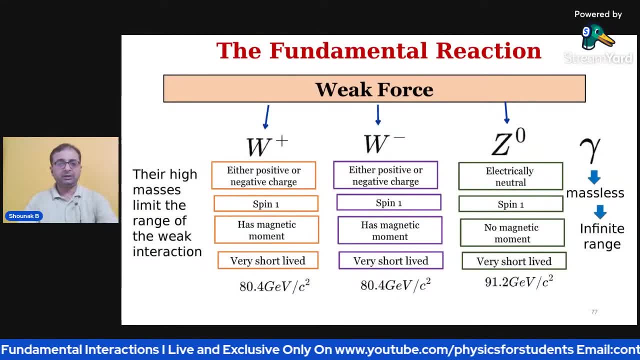 particles, alpha, beta and gamma. and this beta decay was already proposed by Enrico Fermi and later it was united by Stephen Weidman's Salam model. Okay, here is a kind of a summary of what is called the weak force or the weak interaction. So in weak interaction, as you can see, fermions can. 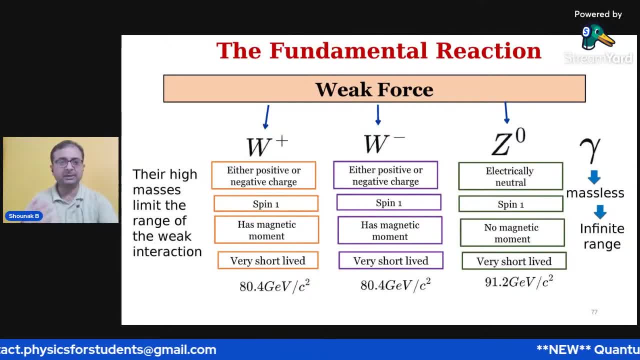 exchange three types of forces. So weak force is basically taking place with exchange with three types of forces. One is W plus, W minus and Z bosons. So the masses of these bosons obviously are far, far greater than the mass of the proton and neutron. 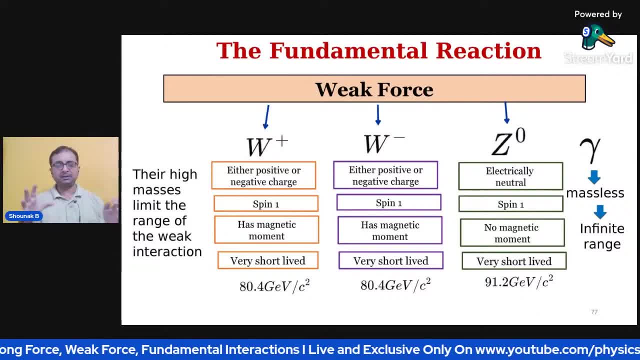 Obviously, proton and neutron do have a mass, but the masses of these bosons are far greater. Now, in fact, the term actually we called weak, it is because its field strengths are, over any set of distances, typically several orders of magnitude less than that of electromagnetic force. So if you 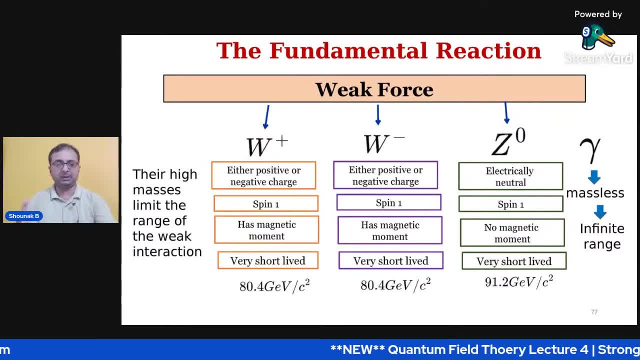 consider the electromagnetic force to be at a certain distance. it is much lesser. So that is why we call it as a weak force. So the, I would say, the higher masses limit the range of the weak force And then, by contrast, you can see if you take a photon, which is the force carrier of the 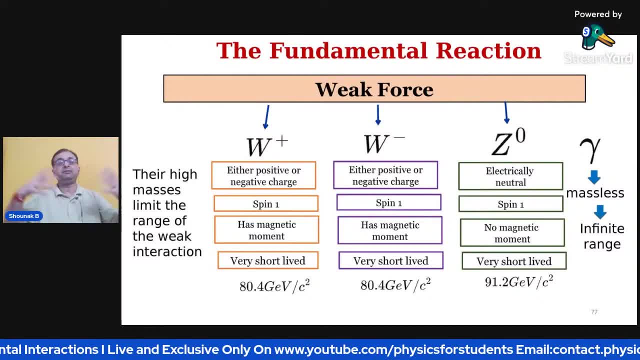 electromagnetic force. it has got zero mass, consistent with infinite range of electromagnetism, And we have, in search of the graviton hypothetical which is expected to have a zero mass. So here you can see W plus which has got either a positive or a negative spin, one as magnetic etc. And I've 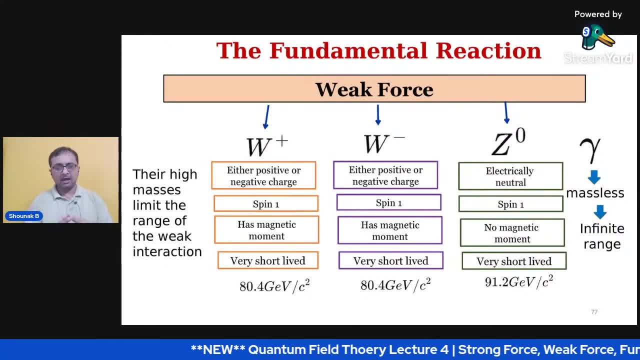 just given the giga electron volt, the values. The photon is massless. It has got infinite range. It can travel up to anything Z zero. bosons are electrically neutral. They have a spin one. right, Remember, these are the spin one. This has also got a spin one and W minus also got a spin one. So 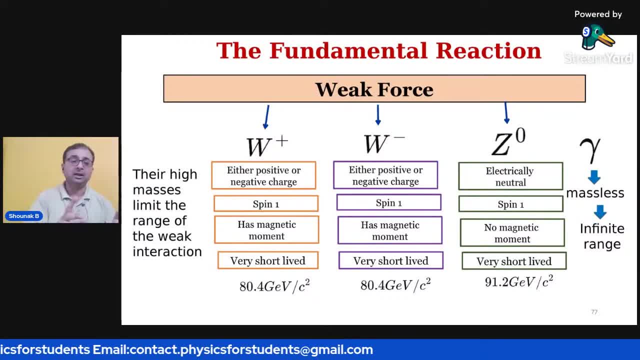 that means these weak forces, because they got have the spin one. that means they are a fermion. Remember, if you, if you go back to my previous class- I mean to say if you go back to my previous classes- I have explained the integer positive, integer, bosons, and then the 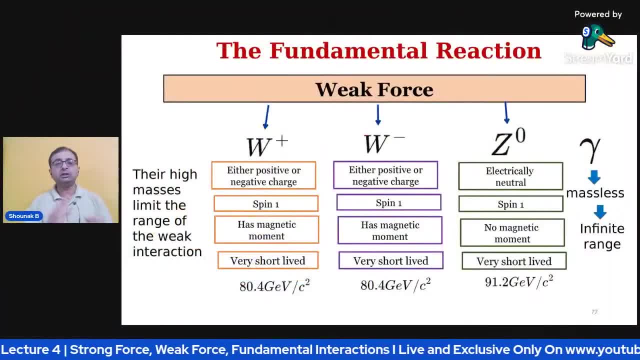 fermions, etc. which has a spin half, which have a spin minus. So all these are very important to understand. Now you can see that the weak force is basically interacting with that of the, you know, with the W plus, W minus and Z zero, And each of them has got a positive integer spin. that is a 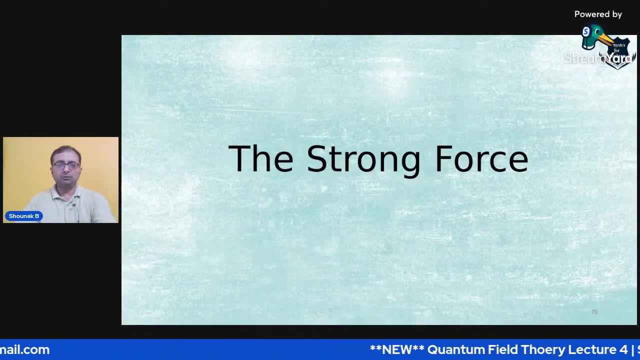 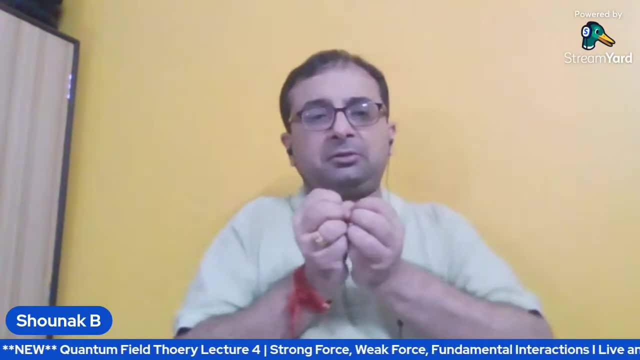 spin one. Okay, now we come to what we, which is known as the strong force. Remember strong force and weak force. It is very simple. The weak force actually is responsible for the decay, So it is the alpha, beta and the gamma particle which is 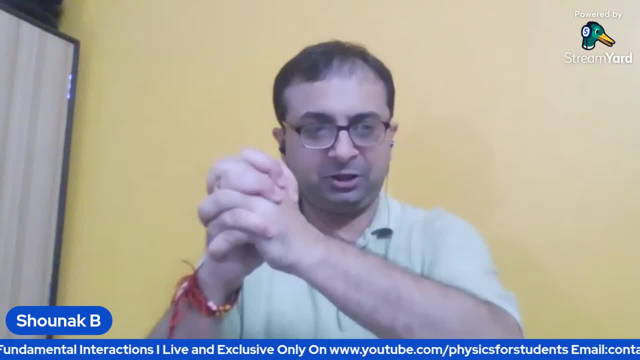 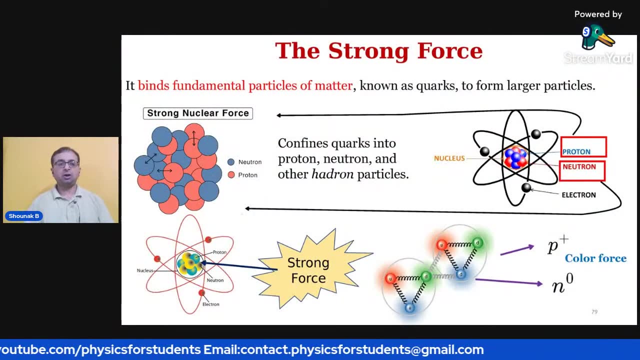 decay, and strong will be called a strong bonding. We have friendship between us, So strong force are those which are keeping the atoms binded together. Okay, so the strong force, as you can see it, binds fundamental particles of matter together and they form up what we call the. 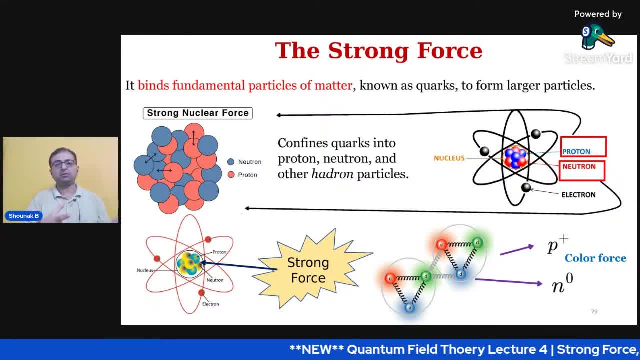 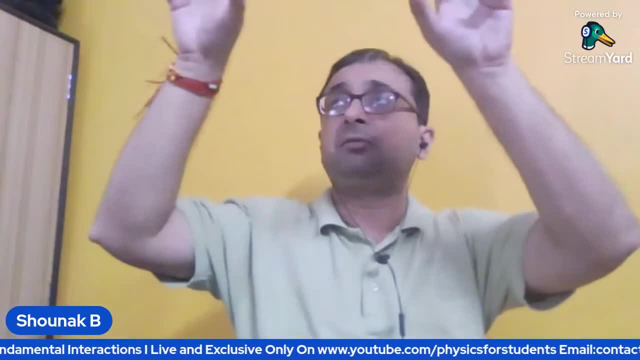 nuclear. So the strong interaction or strong force confines quarks into proton, neutron and neutron formation. If you go back again to my previous classes yesterday also, I draw it on sideboard, a kind of a hierarchical diagram that this you have to be quarks, the leptons and then 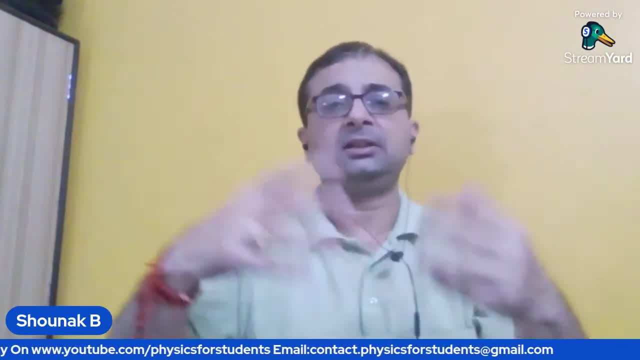 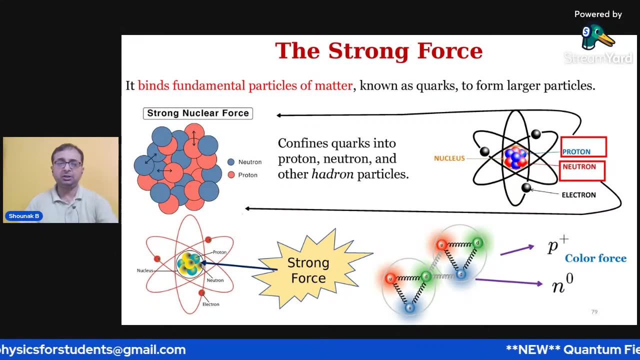 they form the hadrons, Then hadrons are the higher particles, then they are forming the human body, etc. matter everything. So that is how it goes. Now remember that on a larger scale, for about one to three phantometer, if I consider it, is a force carried by mesons that binds protons and neutrons. 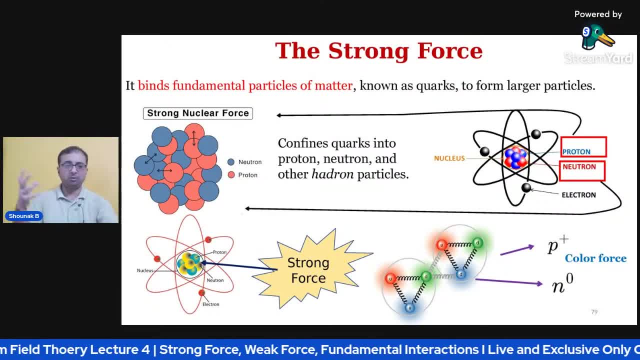 to form the nucleus of an atom. So the nucleus of the atom is formed by finding the forces. So most most important, what is important is that confines quarks into protons and other hadrons and particles. So that is it. So the strong force inherently we can call has such 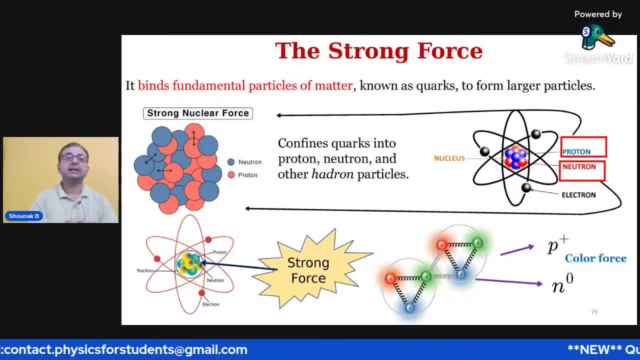 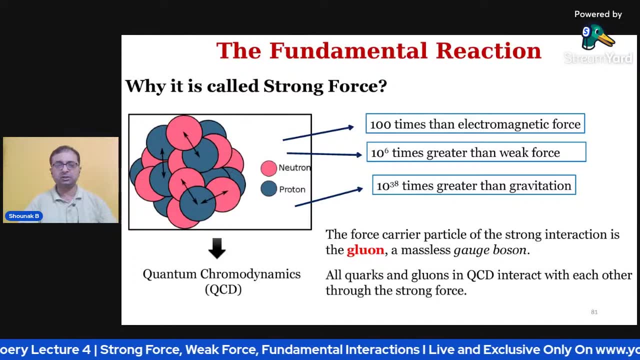 a higher strength, that hadrons bound by the strong force can form new massive particles. These massive particles actually produces mass, gives higher area, and thereby you can say that it is the mass of the matter. Okay, so this is a kind of a quick definition of what is called. what is a? 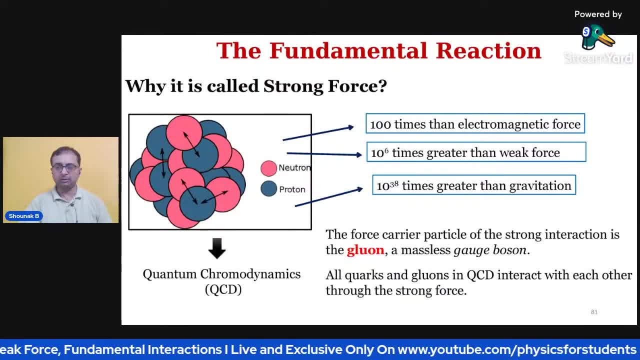 strong force. I mean to say it is quite simple, You can just go through that. It binds fundamental particles together. It is 100 times than the electromagnetic force, 10 to the power, so much times greater than force. 10 to the power, 38 times than that of the gravitational force. So the force. 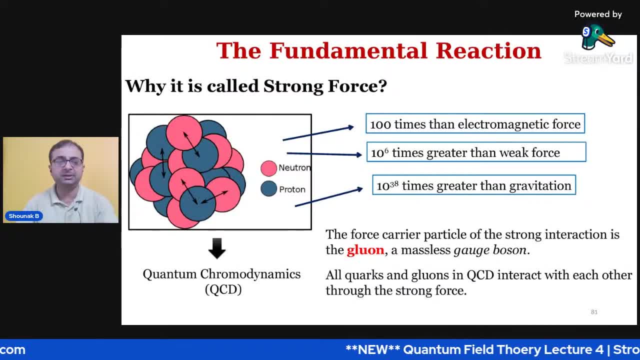 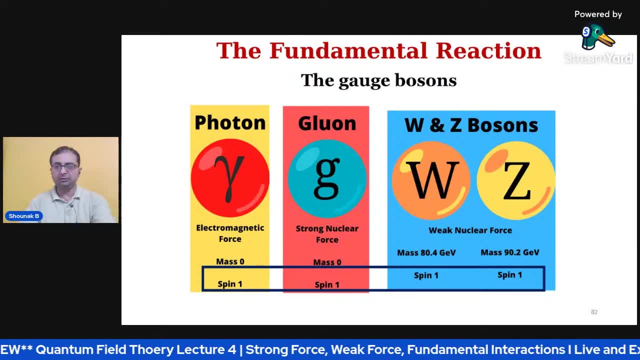 carrier or the particle of the strong interaction, is basically the gluon or the massless bosons. Next I go to this, this part, which is which? okay, I am so sorry, I think I have missed one slide. No, this is fine, Right. So this actually, you know, determines a kind of a summary of what it. 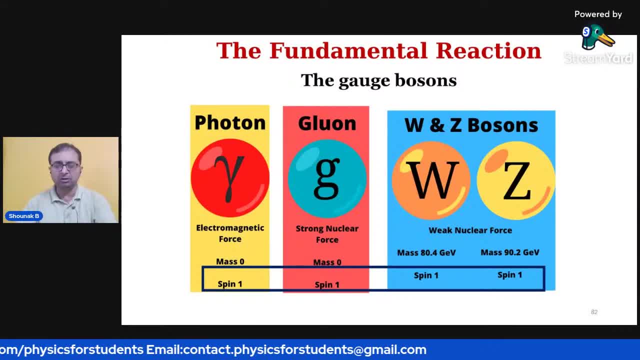 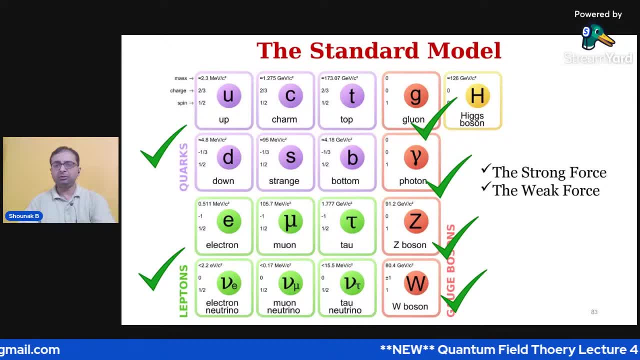 is actually the photon which has got mass zero. Then we have gluons, Those are the strong nuclear force. Then we get W and Z bosons, which is spin one particle, And then now you can see that we have actually explained the standard model. 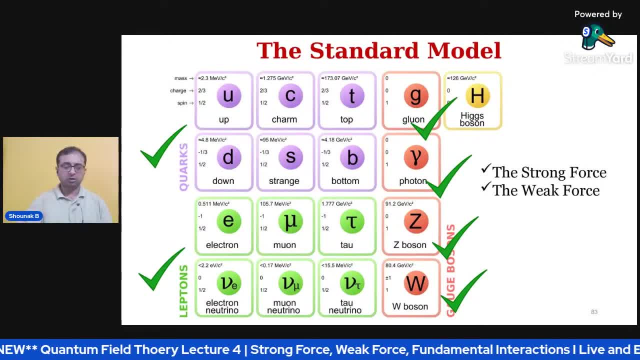 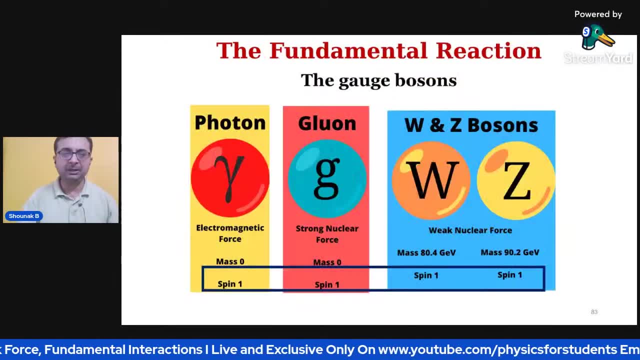 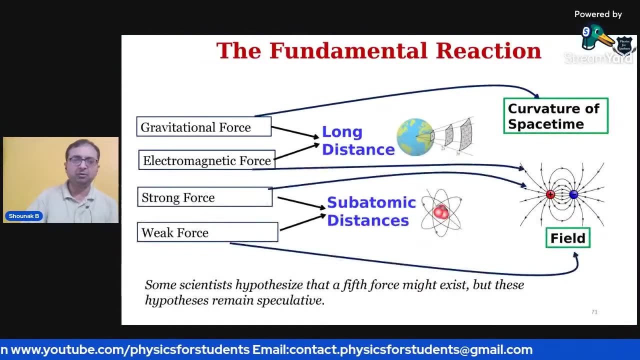 Which is the quarks, the leptons, the photons, the Z bosons, gluons and so on And the gauge bosons, So strong and the weak force together. So this actually completes one part of our lesson. I mean to say starting from the strong force, the fundamental reactions, the weak force. 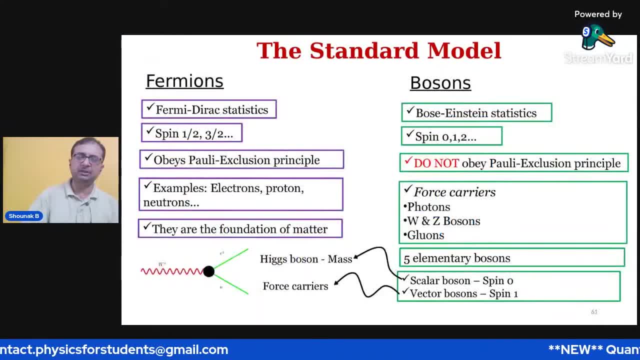 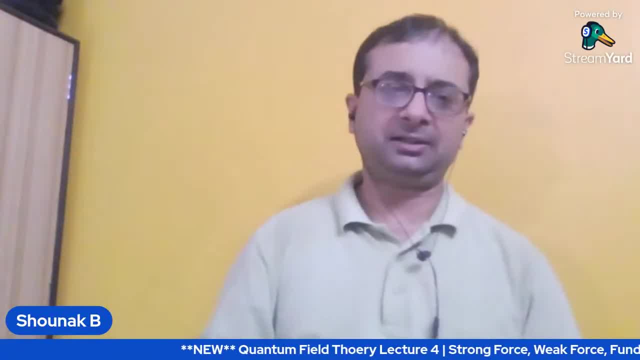 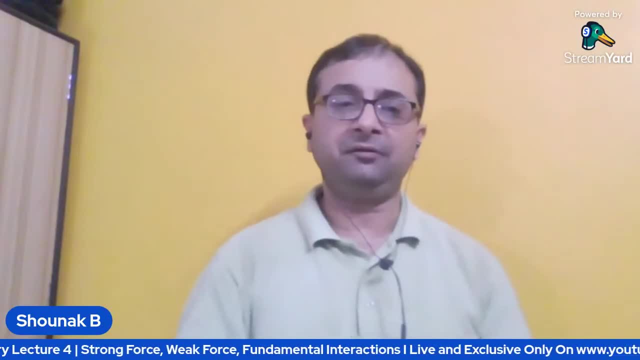 the limitations of the standard model. And if you go back previously, I have covered the standard models, the fermions, bosons, etc. So in the lesson, what we are going to do is that I am going to present some more mathematical ideas, starting with the Lagrangians, which are a very central part of, I would say, quantum. 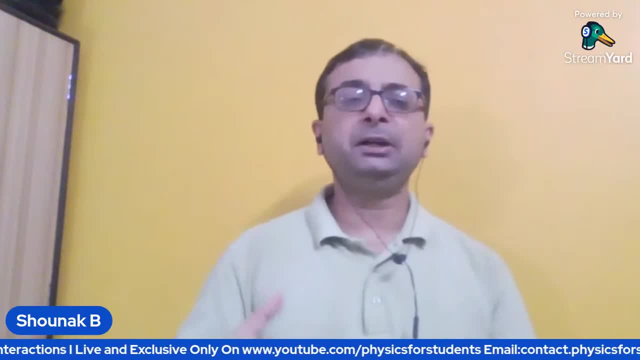 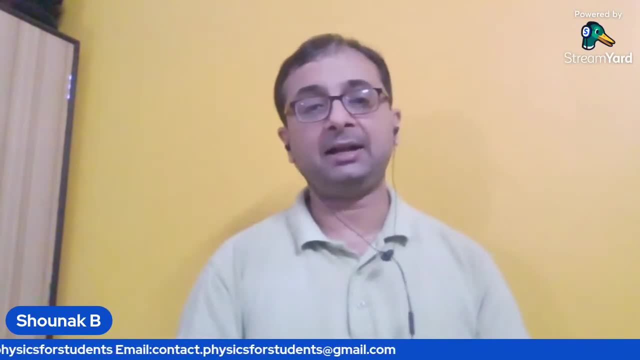 filter or any form of physics, And I am starting up a new series of lessons on what is called general theory of relativity, which would be also a part of this lesson, And it won't be like videos which I make. It will be more mathematical in nature. It will contain equations and going deep. 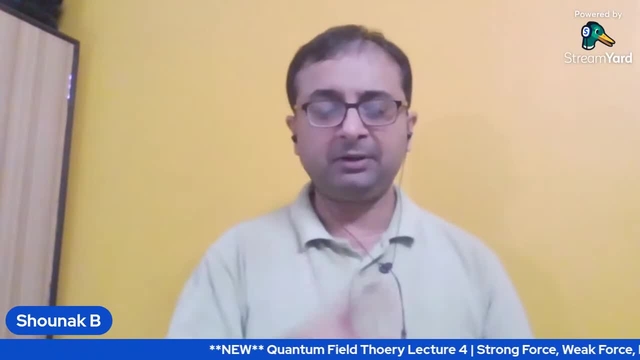 into the complexities of tensors etc. But I will try to come live tomorrow, But I am not sure. Maybe, if it is not tomorrow for sure, for Monday another lesson on quantum field theory. I will quickly brush up and make a kind of an easy. 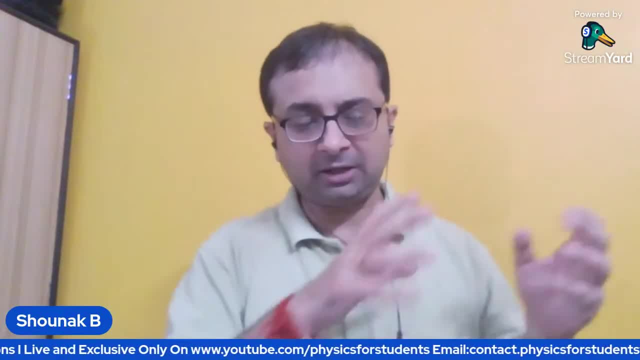 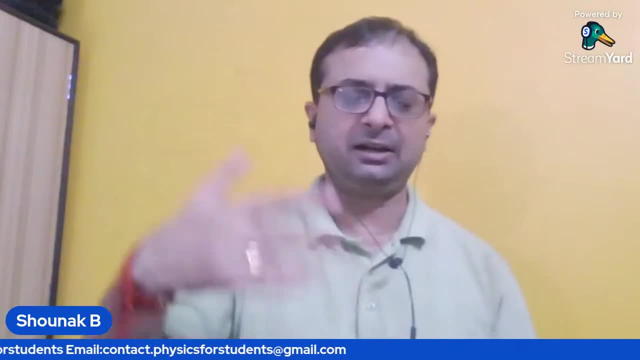 understanding of what are the things that we have learned, starting from the basic to today, And then we will start with the mathematics. We are starting with the Lagrangian formulation, taking the standing waves, complex plane waves, things like that. So this is a re-recording, because live streaming I 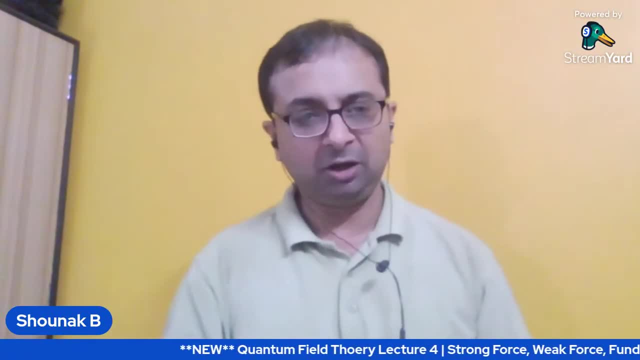 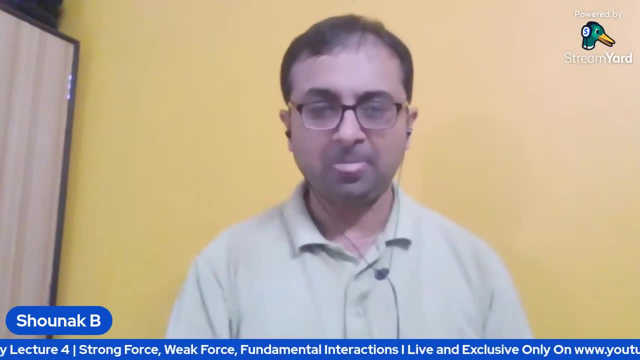 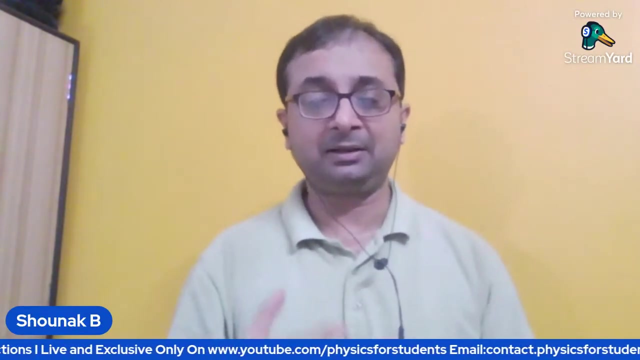 mean to say Because the last video had problems with the audio. I am so sorry, My kind apologies, And I think this video is quite good enough. You can hear my audio video and everything. So next lesson again on quantum field theory, with a new lesson coming up on general theory of relativity, More on the mathematical 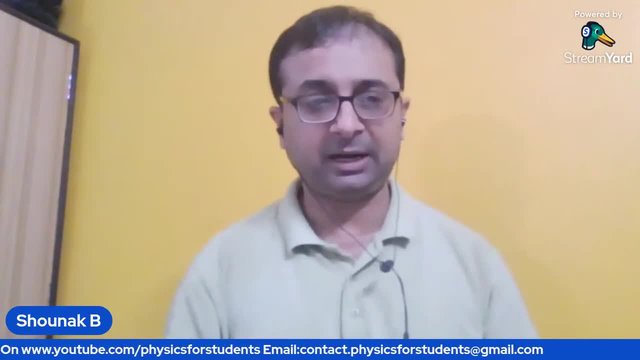 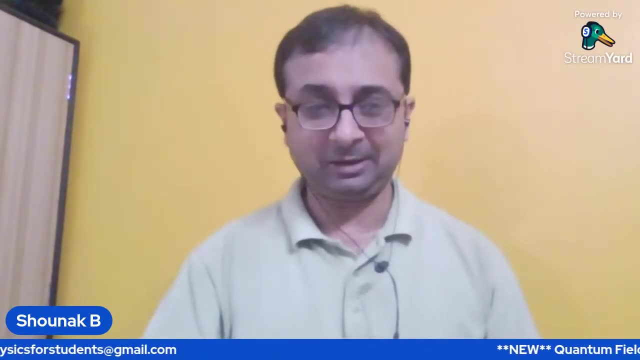 and the real mathematics explaining general theory of relativity right from the beginning. Thank you very much for coming to this live stream and to let me know how it was and how things are going in the comment box. Thank you, A very good evening and I wish you a very